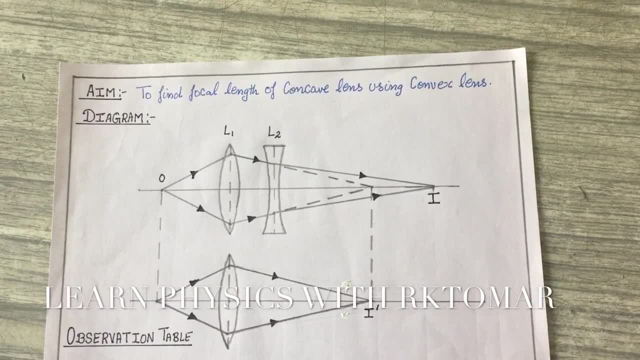 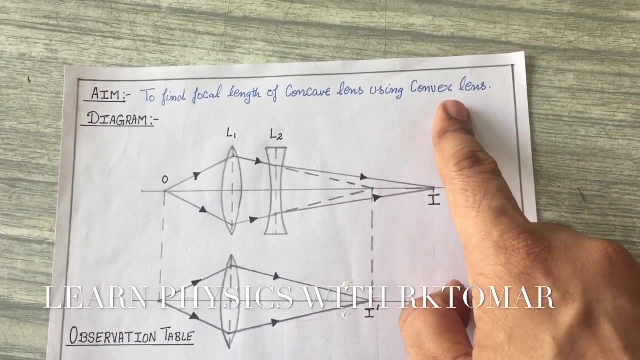 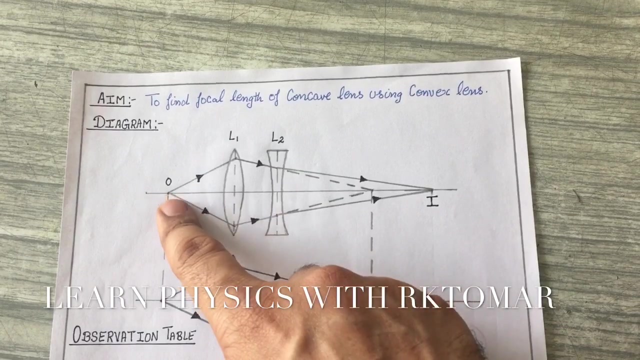 hello everyone. welcome to my youtube channel. learn physics with RG Tomar. In today's video we are going to perform another experiment to find focal length of concave lens using convex lens. As we can see in the diagram, O is the object where we have L1 as convex lens, L2 is concave lens, O is the acting as object. 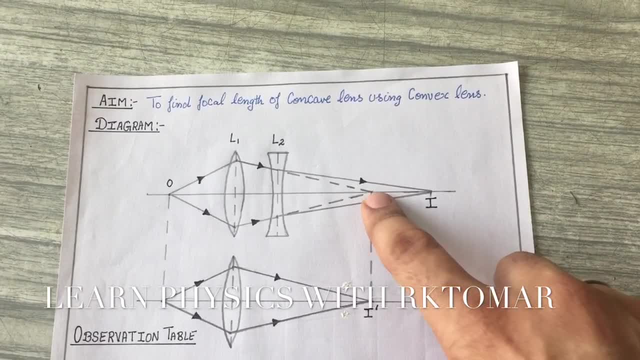 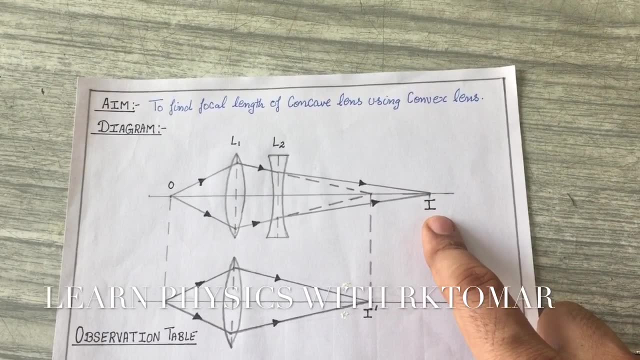 for convex lens, whose image is going to be formed as I dash, and this I dash is acting as the object for concave lens, whose final image is going to be formed as I, So the final image of the whole system is I. Now you have to see the 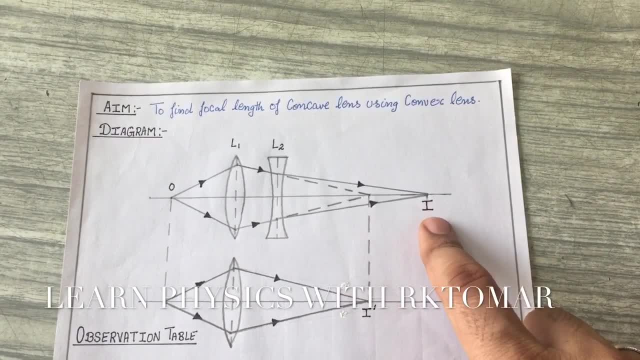 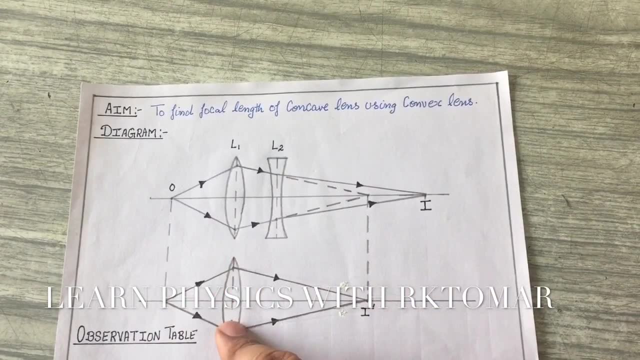 O object needle on the optical bench and on the other side you have to focus the other image needle on it and we will get the position of I Now how to find I dash in this. So for that we will analyze the second diagram Now in this: 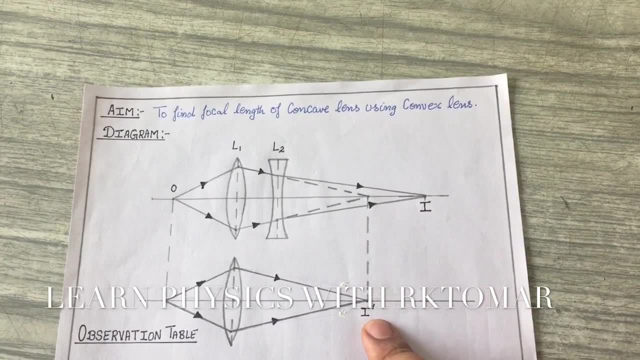 we will remove the concave lens from the optical bench. The position of the object needle will be the same as that of the concave lens. Now we will see how to find the focus of the object needle. Now we will see how to find the focus of the object needle. Now you have to pull the object needle out. 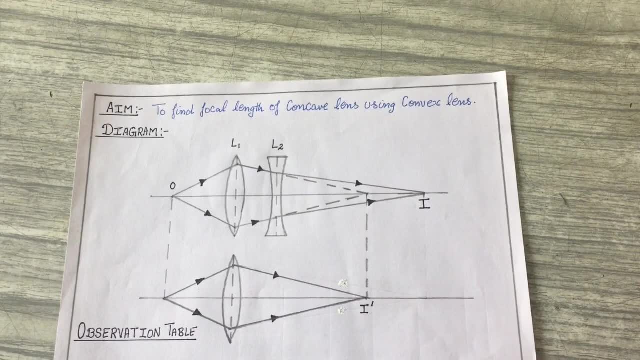 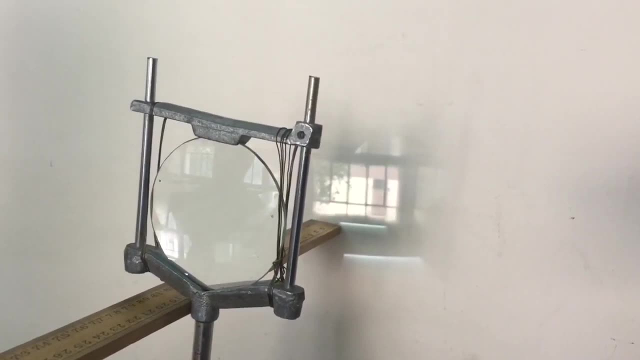 of the object needle, and you will see that object is now in the box. Now that object is now in the box, you can see the object needle remains there. the convex lens remains there too. Now you have to focus it from the other side and we will get the I dash. So first of all, now let's remove the rough focal. 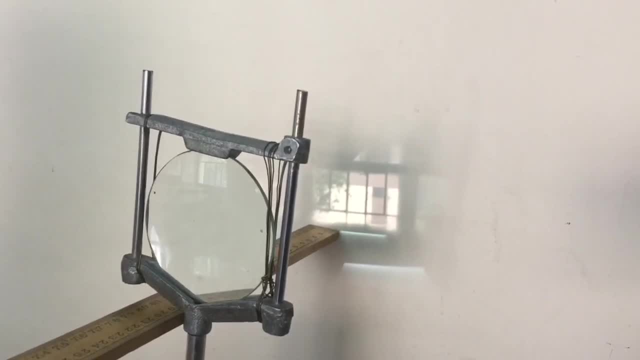 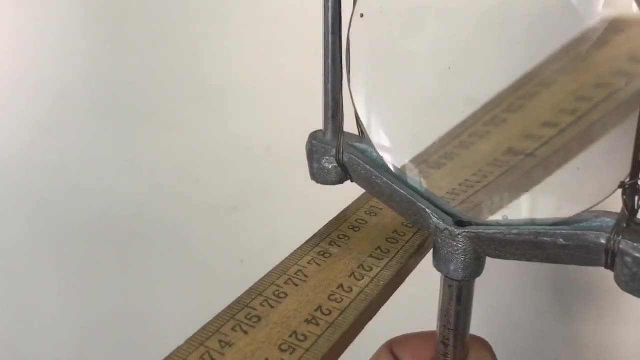 length of convex lens. So now I am trying to focus an image of a distant tree on the wall. See, the wall should be seen carefully first. you see a fade image is being made and roughly the distance is around 20 cm. so the rough focal length of this convex lens is 20 cm. 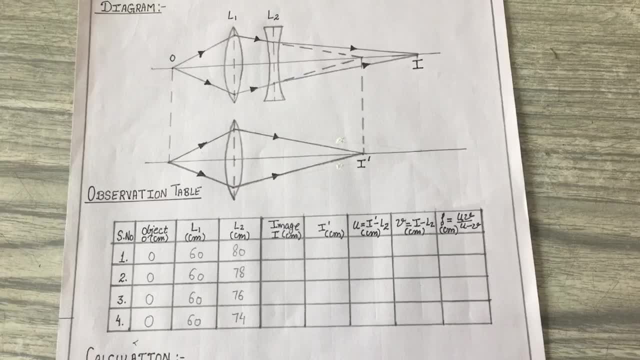 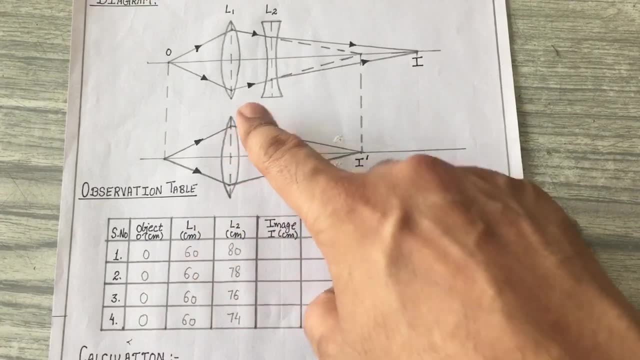 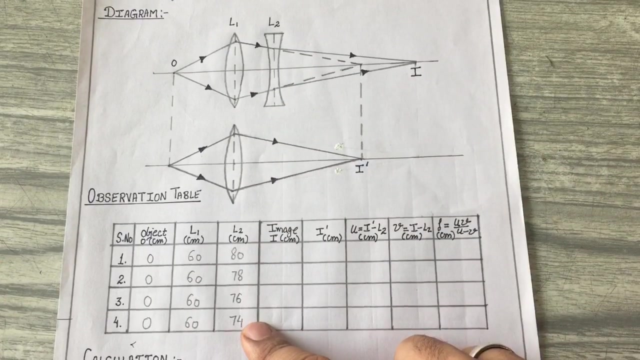 now let's see the observation table. here I have fixed the position of the object needle, which will always be at 0 cm. then I have written the position of L1 and L2. position will also vary in this experiment. we have to change the gap between L1 and L2. 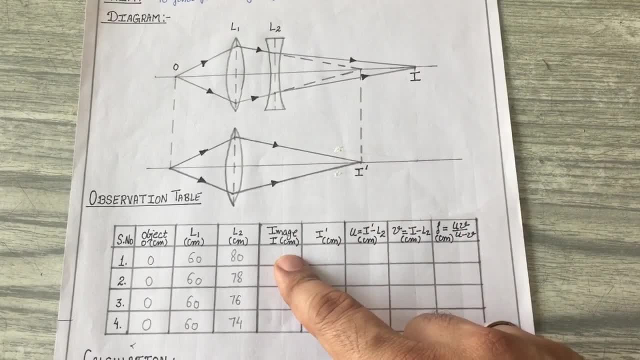 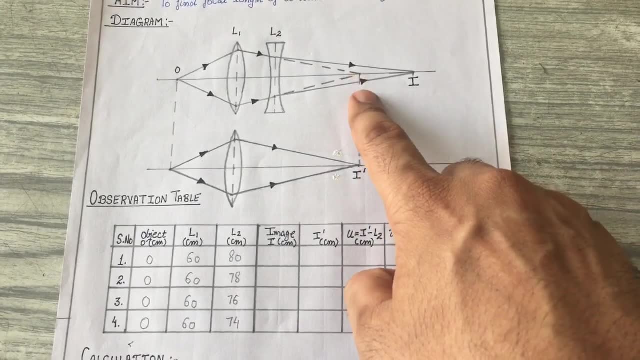 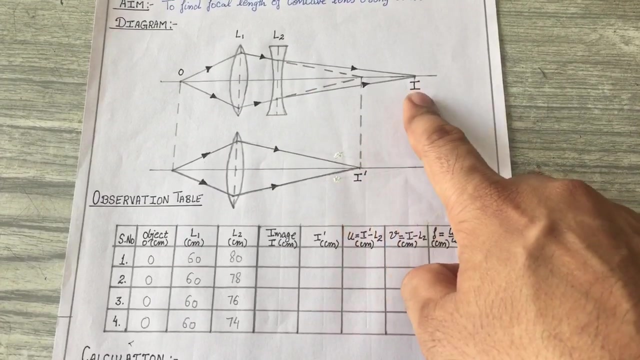 and for different, different positions, you have to find the values of I and I' and, as I told you earlier, for the whole system, I is the final image and I' is working as an object for the concave lens, so the distance between I' and the concave lens. 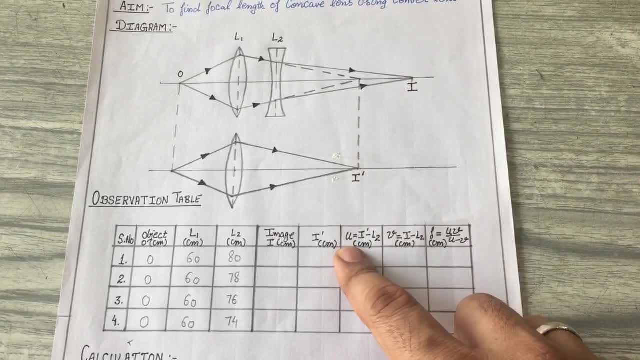 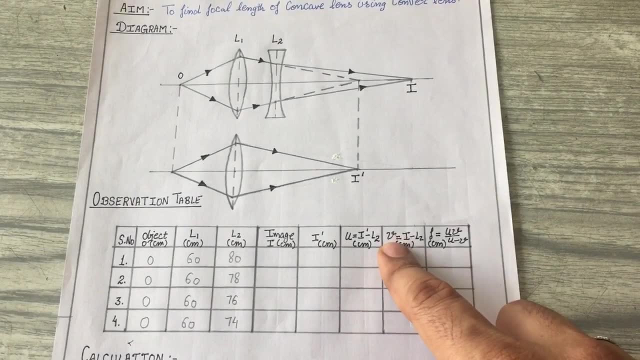 will be U, which is the object distance, and the distance between I and the concave lens, which you can see in the observation table between L2 and I will be V. so you just have to find the values of U and V and then we will use the thin lens formula. 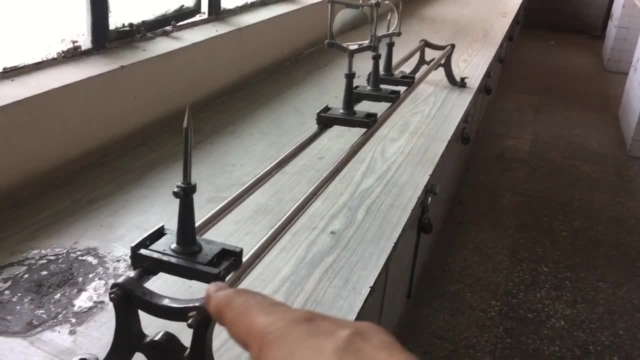 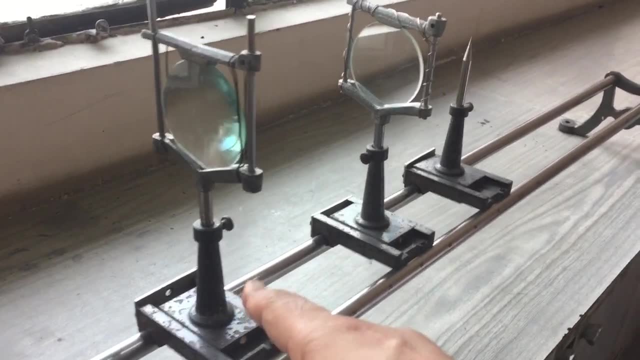 and then we will find the focal length for every case, and this is our experimental setup. so, on the optical bench you can see, first was the object needle, this is the convex lens, and after that we have kept the concave lens and the second needle you are seeing. 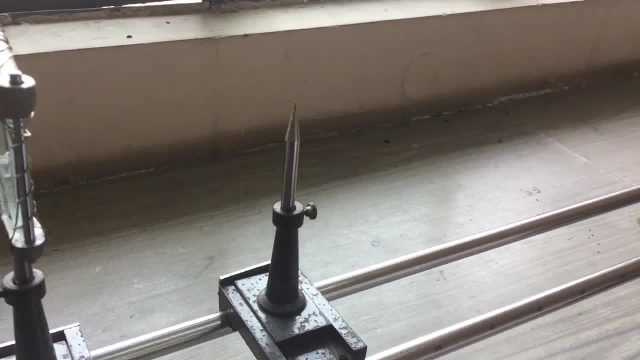 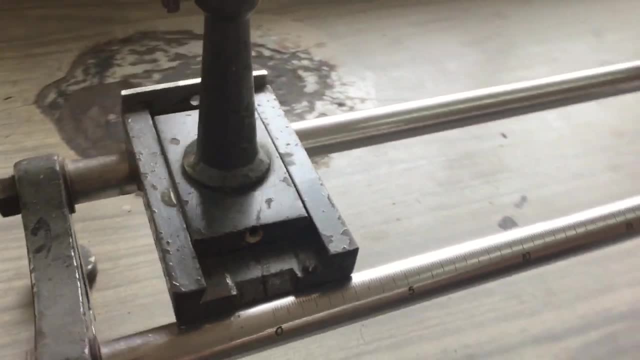 this will be acting as the image which we saw in the diagram. it will be I when the concave lens is also there. when the concave lens is removed, then it will be I'. the position of the object needle you are seeing is at 0 cm. 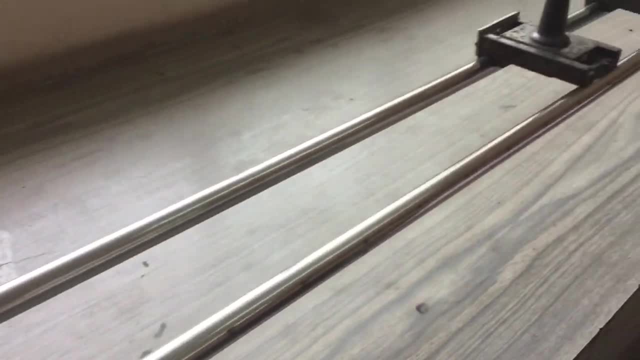 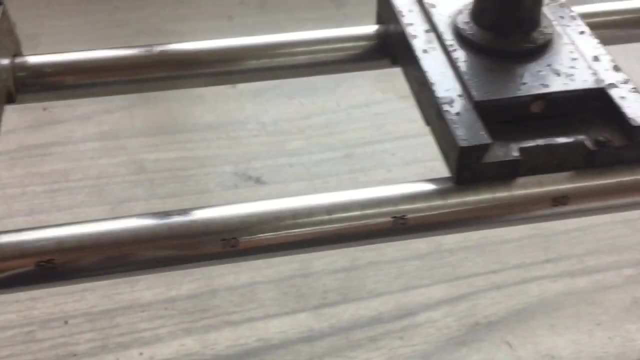 which we will always keep fixed. let's see the position of the convex lens. as I told you in the observation table, we have fixed it at the reading of 60 cm. now our concave lens is at 80 cm, which we have to vary again and again. 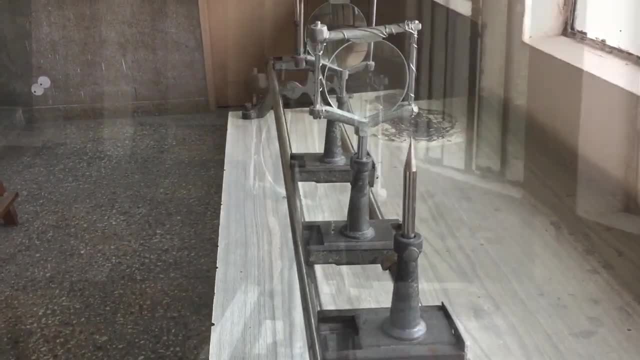 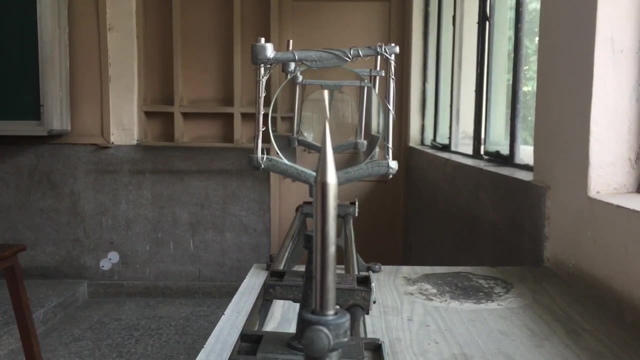 and from this side, you have to vary the position of the image needle and you have to see the image needle of the object which you are seeing through. the lens should be at the tip of the image needle, as I told you in the previous videos also, that there should be no parallax error. 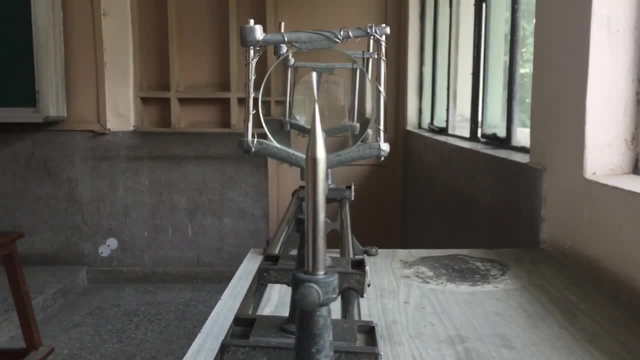 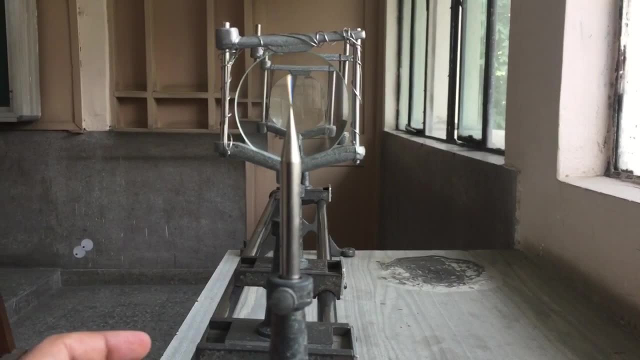 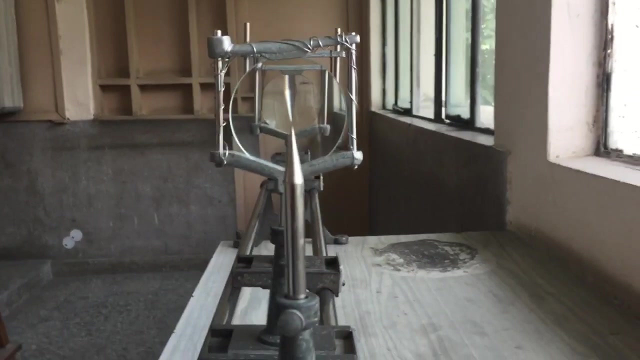 which means you have to move your left or right eye and you have to see that the image needle and the object needle should move together. so, as you can see, there is no parallax error at this time. so guys, watch this carefully, and while doing this you have to be very careful. 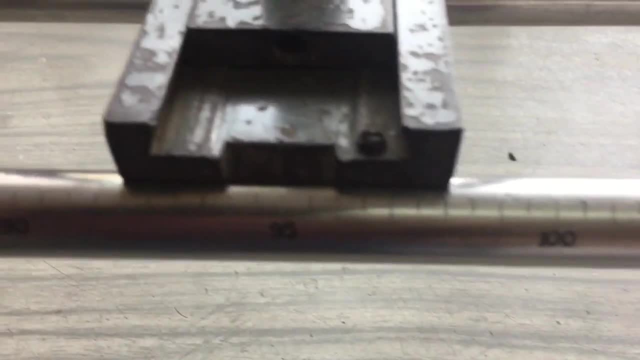 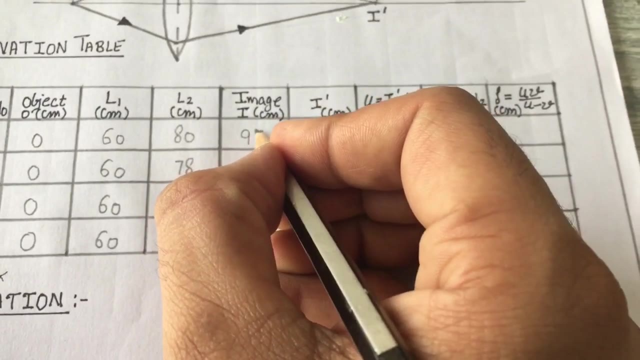 now we will note the reading, and the reading is approximately 95 cm, which is our first reading. now let's write this in the observation table: that the position of the image is 95 cm. now we have to take out the eye dash and for that we have to. 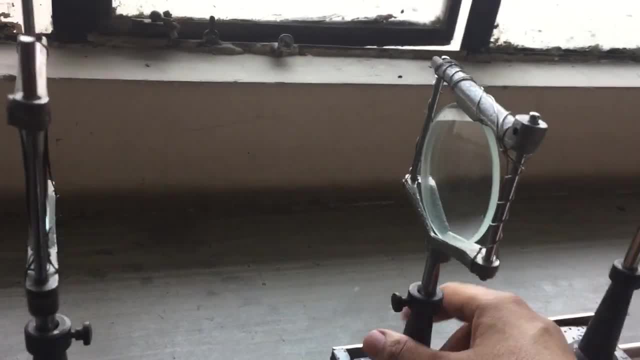 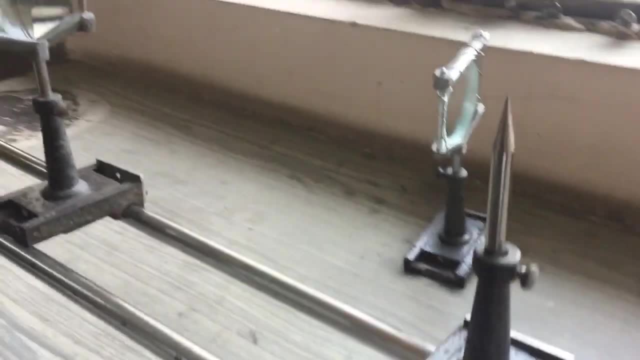 remove the concave lens from the optical band. so now we are removing the concave lens from the optical band, we don't have to change the position of the convex lens and the object needle. now you have to adjust the image needle again so that the image of the object 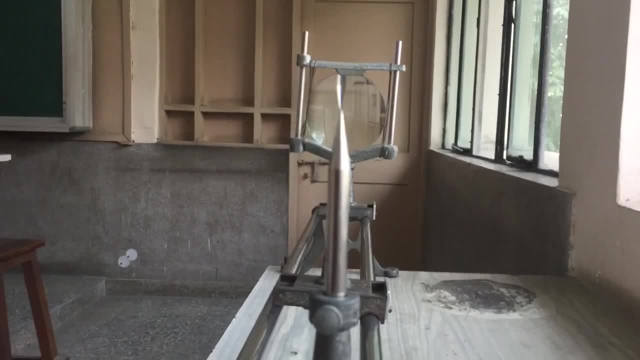 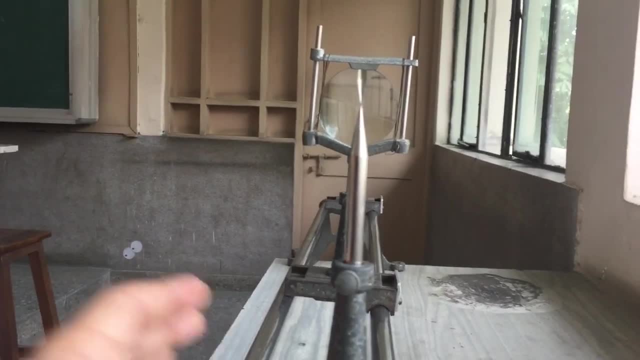 which will be seen through the convex lens, will be the same as the image needle and the angle of the eye dash should coincide at the tip of the eye dash. and yes, this time also there should be no parallax error. so, as you can see, there is no parallax error. 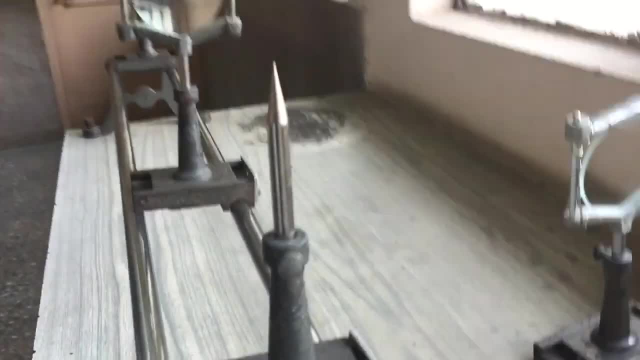 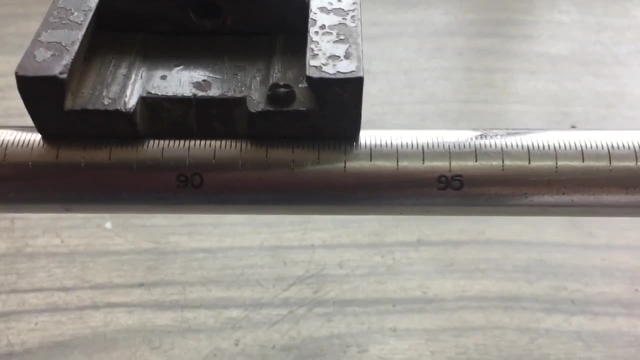 for this you have to make some adjustments, and when you do it in the beginning, it takes a little more time. so practice it so that it moves quickly. now let's note the reading, and the reading is approximately 90 cm, so let's take this in the observation table. 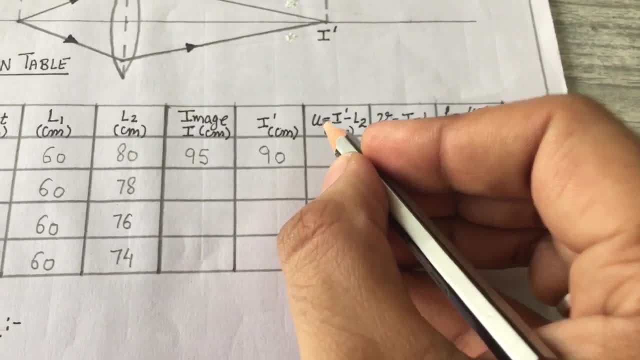 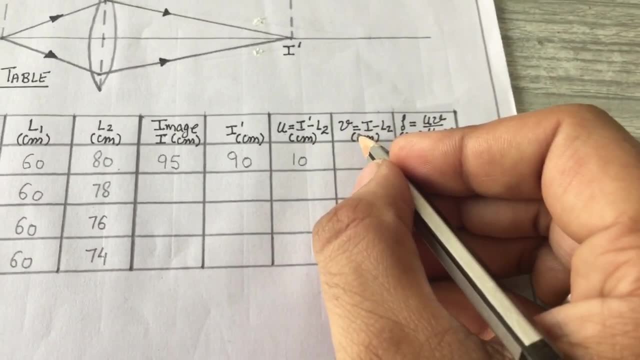 90 cm. now you can see in the table, if we take out the U, it will be the gap between the eye, dash and L2, which is 10 cm. similarly, we will take out the V, which is the gap between the eye and L2, and that is 15 cm. 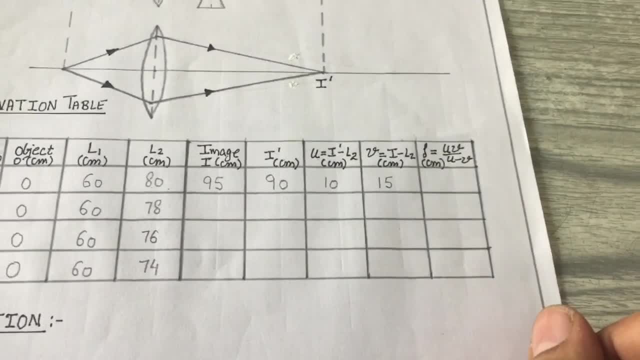 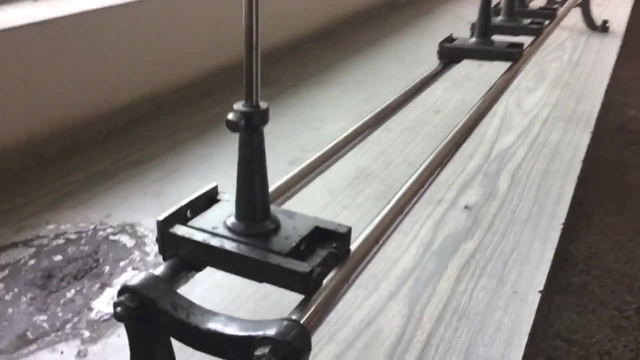 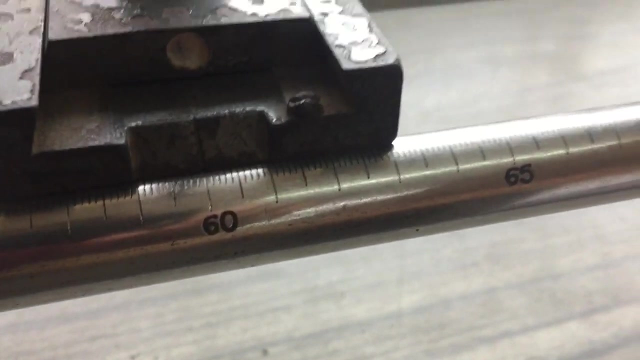 similarly. now you use the thin lens formula and the value will come out similarly. you have to note the rest of the readings. let's do that too. so I have seen that the object is still at 0 cm. convex lens is still at 60 cm, this time. 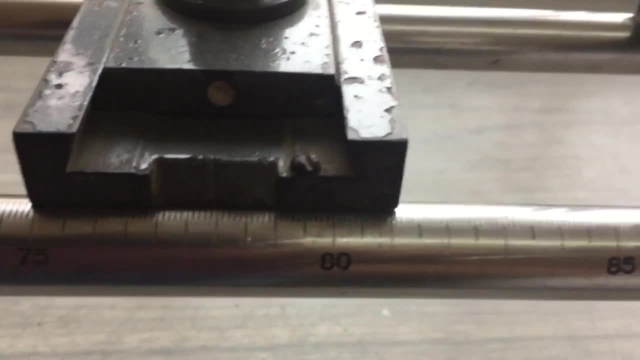 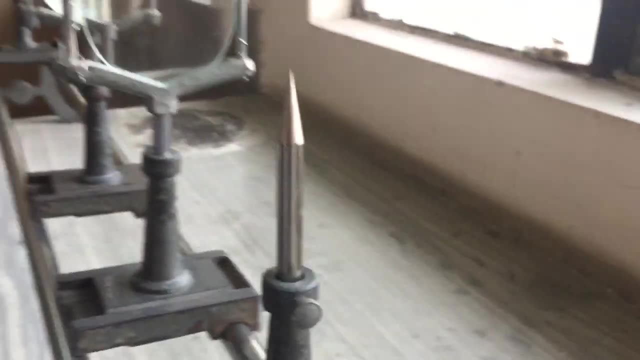 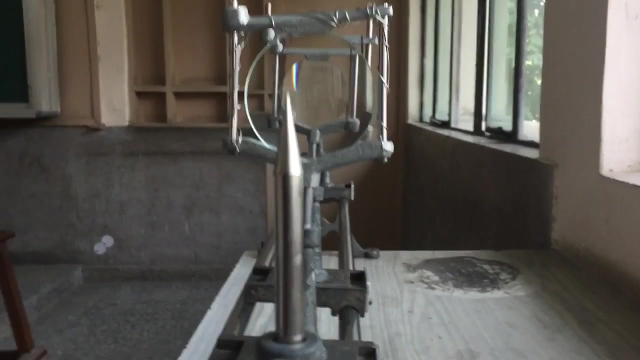 I have to shift the position of the concave lens, and we have shifted it by 2 cm, as we had written in the observation table. then again, you have to vary the position of the image needle such that the image of the object needle coincides with the image needle. 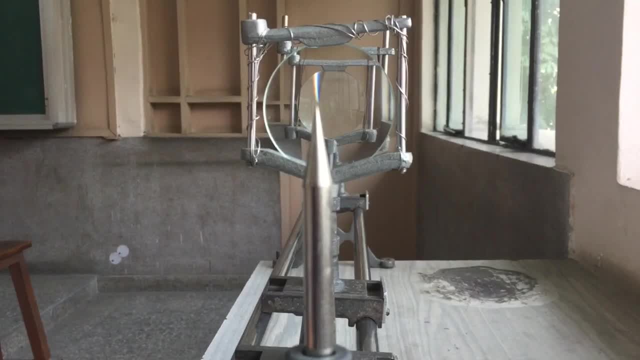 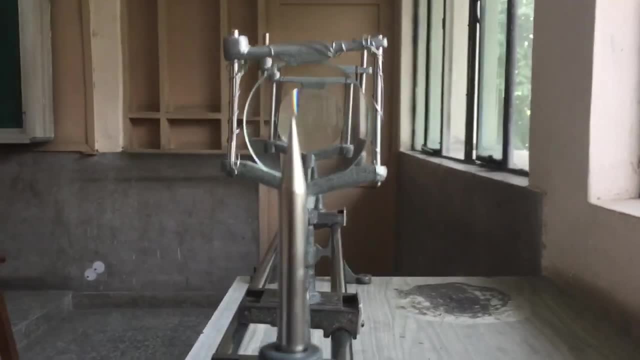 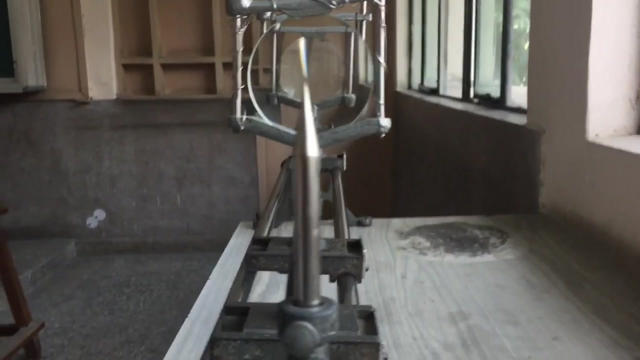 parallax error is not there this time. see, I am adjusting and trying to remove the parallax error. now it is going to be removed and it is almost done. now let's note the reading of this time, and that is approximately 96.5 cm. now we have to write. 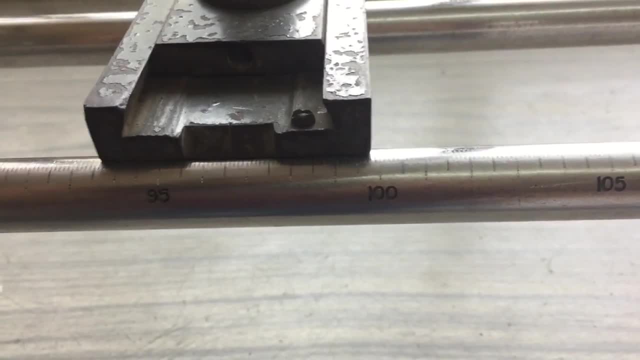 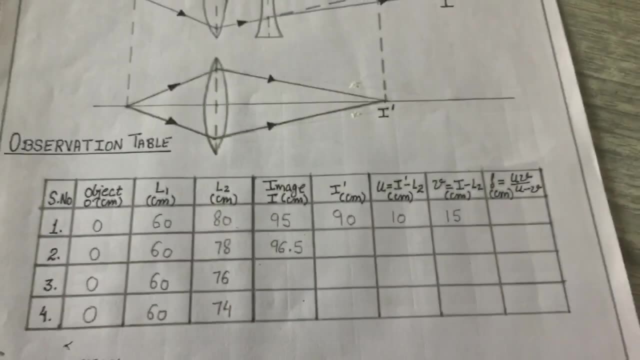 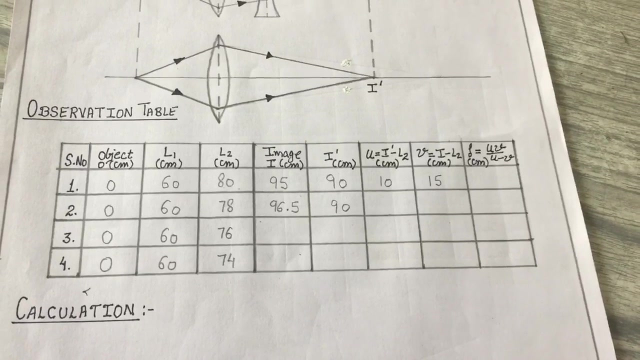 the same reading in our observation table. now our reading is 96.5 cm and now we have to remove the concave lens. so the object needle and convex lens are still there, so the eye dash will remain the same, and that is 90 cm now. in the same way.